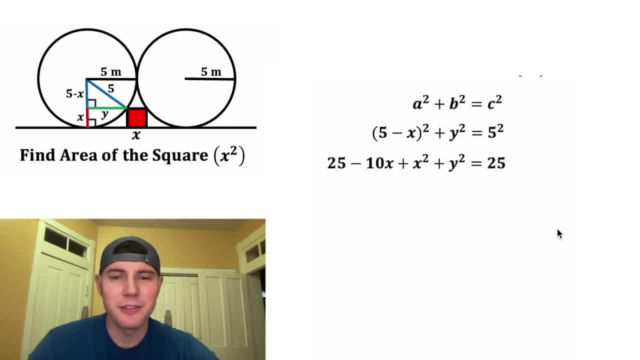 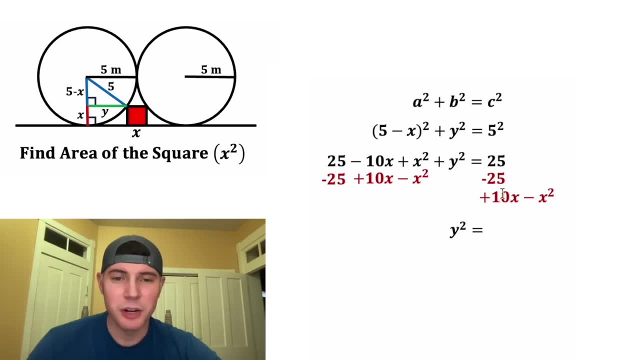 y squared and it'll be equal to five squared, which is 25.. And then we can subtract 25 from both sides and we can also subtract the rest of this stuff from both sides. On the left-hand side we only have y squared and on the right-hand side we have 10x squared. 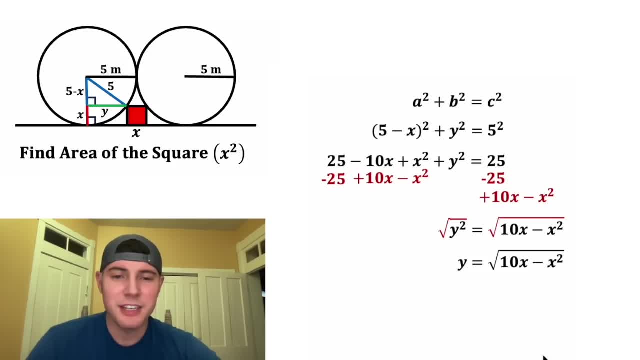 minus x squared. After we square root both sides, we have y is equal to the square root of 10x minus x squared. And now we can clean things up a little bit. Let's scoot this over here and let's duplicate the y over here. Now this distance is going to be equal to this distance. so we know. 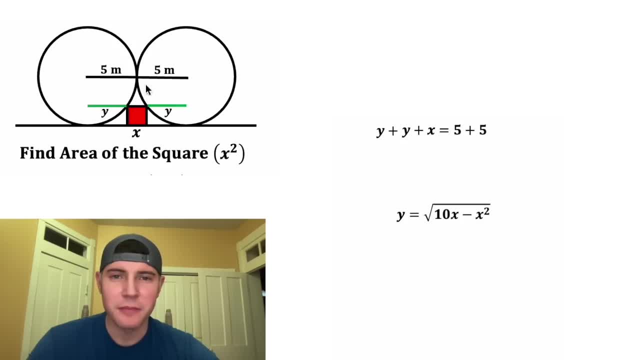 that y plus x plus y is equal to five plus five. And we can clean this up a little bit: y plus y is 2y, and five plus five is 10.. And now we know that y is equal to the square root of 10x minus. 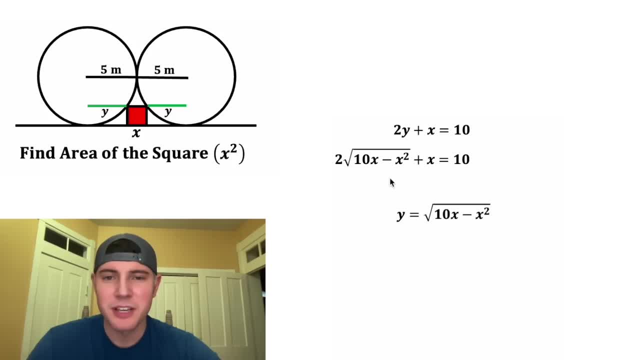 x squared. So in the place of this y we can plug in square root of 10x minus x squared. And now we just got to solve for x. We can subtract x from both sides. That'll give us two times the square root of 10x minus x squared is. 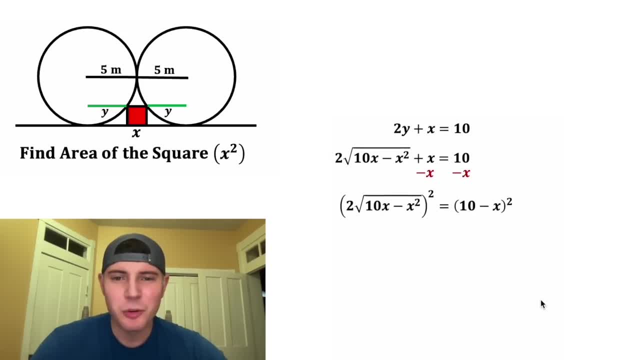 equal to 10 minus x, And then we can square both sides of the equation. This square will distribute to both of these, so we have two squared and then we have this stuff squared. Two squared is equal to four and this square, root and this square are going to cancel each other out, And then 10 minus. 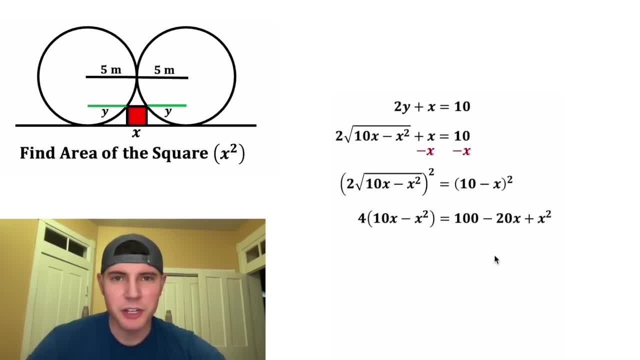 x squared means this times this: and it ends up being 100 minus 20x plus x squared. Then we can distribute this square root of 10x minus x squared to the square root of 10x minus x squared. It'll give us 40x minus 4x squared, And then we can subtract this stuff from both sides. 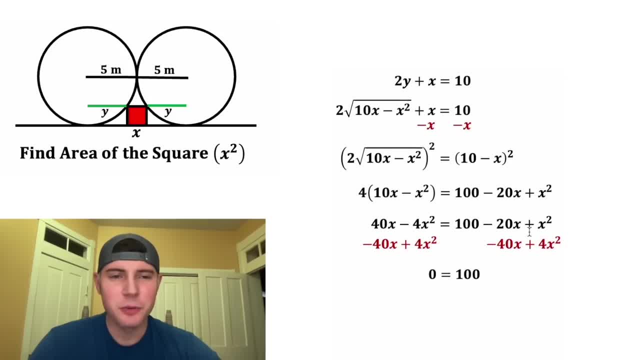 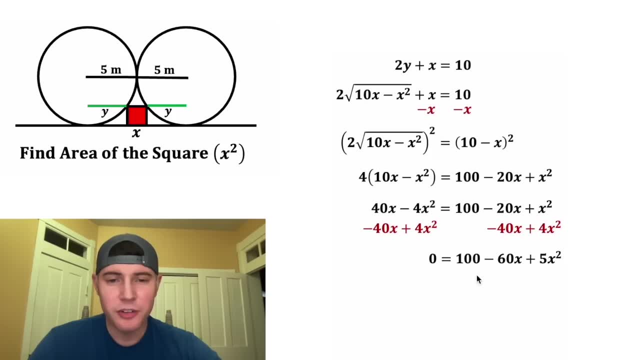 so we can set it all equal to zero. Let's bring down the 100.. Negative 20x minus 40x is negative 60x, and x squared plus 4x squared is 5x squared. All three of these coefficients are divisible by. 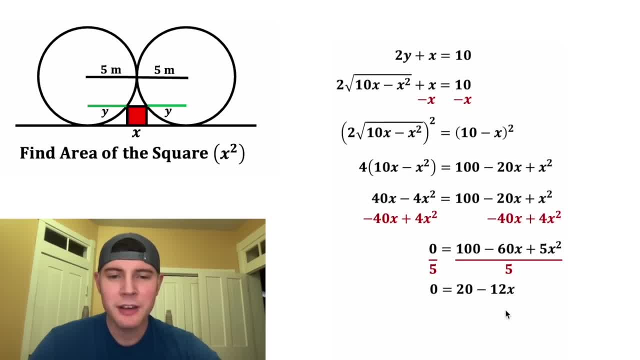 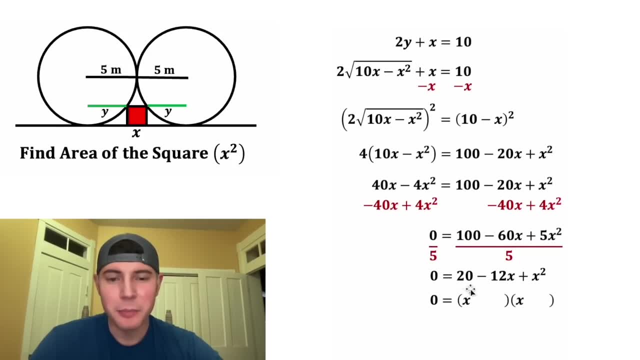 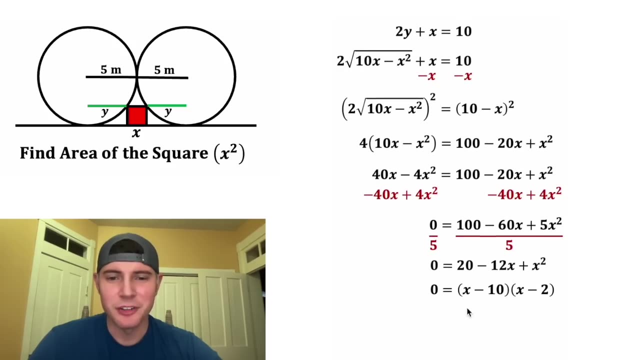 five. so let's do that. We end up with zero equals 20 minus 12x, plus x squared, And then we can factor this: We need two numbers that add to negative 12 and multiply to positive 20.. Well, it's going to be negative 10 and negative 2. So we have x minus 10 times x minus 2 equals zero. That 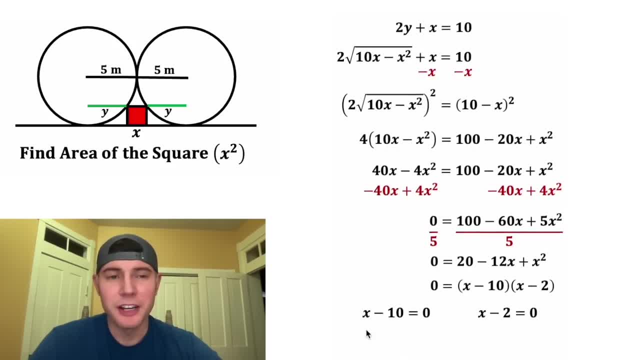 means that either this equals zero or this equals zero. So for x minus 10 equals zero. we can add 10 to both sides and we get x equals 10.. What we can see right here, since the radius is 5, there's no